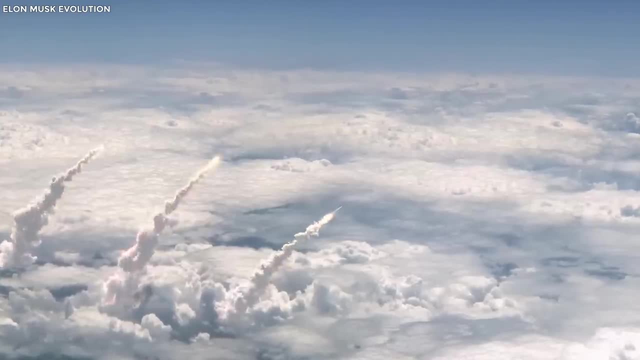 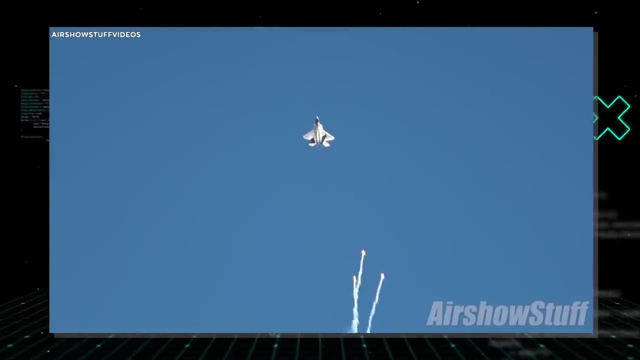 superior fighting equipment. The sky is where much of the competition is these days, thanks to the unique features of aerial warfare. World powers are countering threats from the sky with their own fighter jets, which are becoming more powerful and sophisticated, One of the undisputed 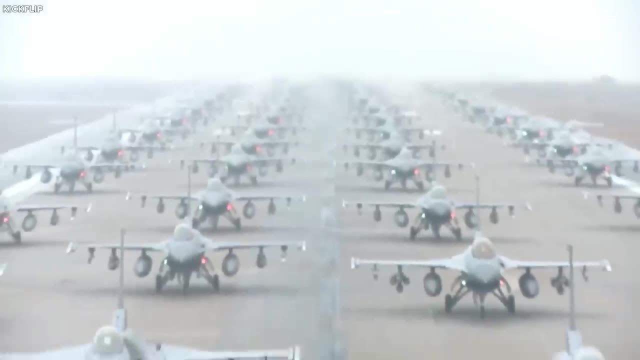 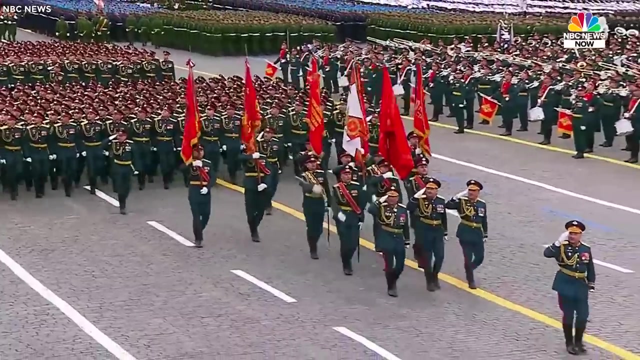 leaders in the arms race is the United States, and a good chunk of its annual budget goes to strengthening its warfare capabilities. It is kept on its toes by Russia, its arch-enemy on the global scene. However, one of the unique features of the US arms industry is that it 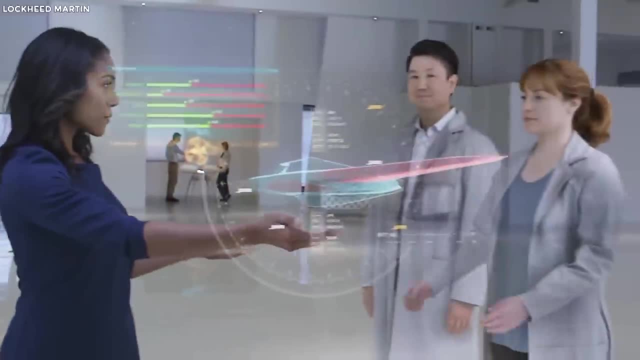 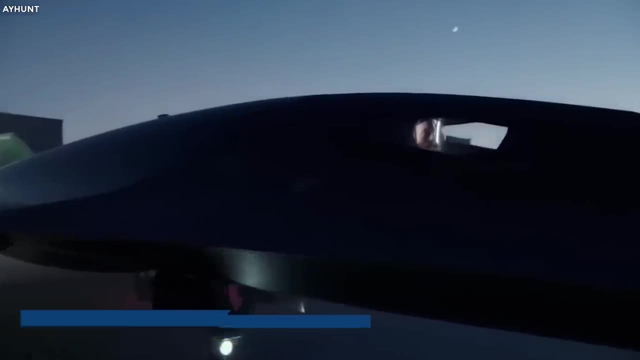 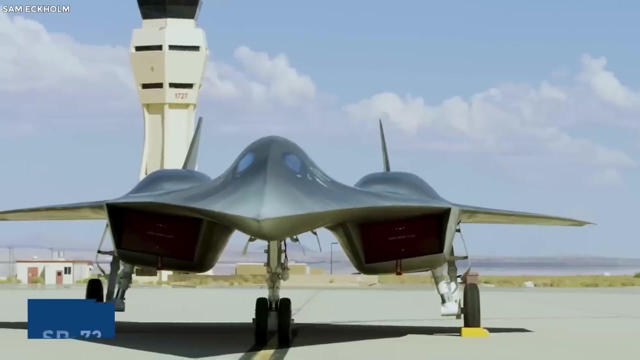 gets lots of innovations from the private sector. One such private sector company is Lockheed Martin, and it's currently developing the top-secret SR-72 high-performance aircraft. If an airplane needs a predecessor to be successful, it couldn't have gotten anything better than the SR-71 Blackbird. With the new SR-72,, Lockheed is building on the success of 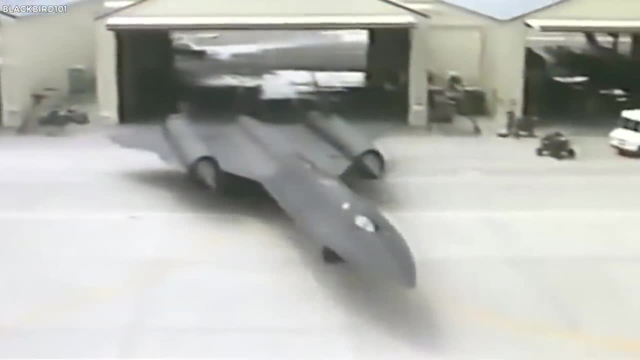 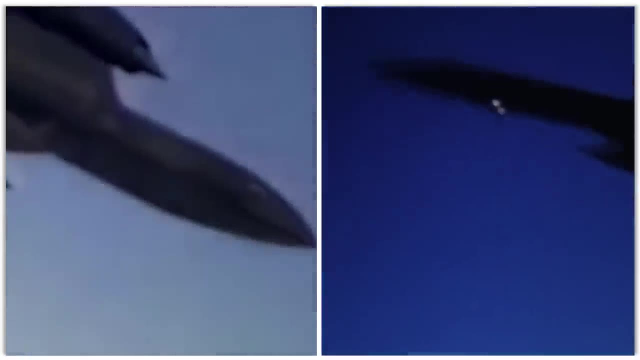 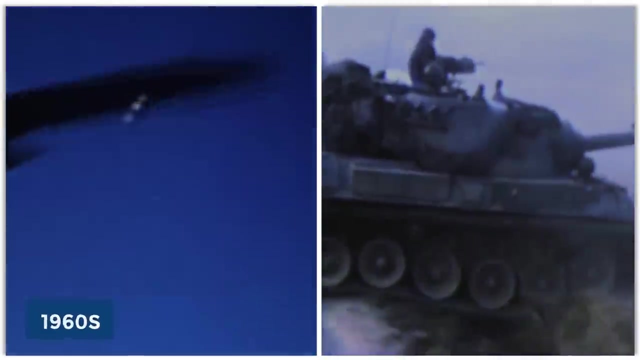 the SR-71.. The Lockheed SR-71 Blackbird remains the fastest and highest-flying jet aircraft in history. It has flown higher than any other and set the world record for sustained altitude flight flying at 85,000mph. Blackbird was developed in the 1960s during the Cold War, as a high-flying reconnaissance jet. 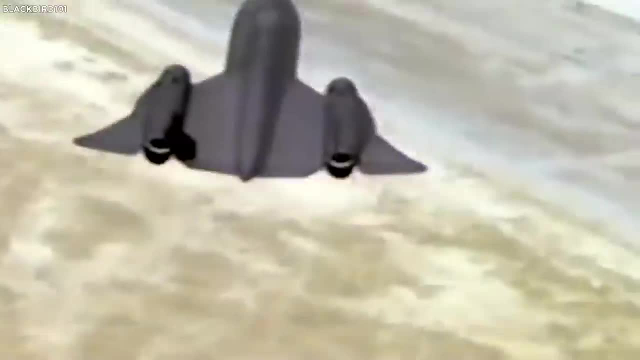 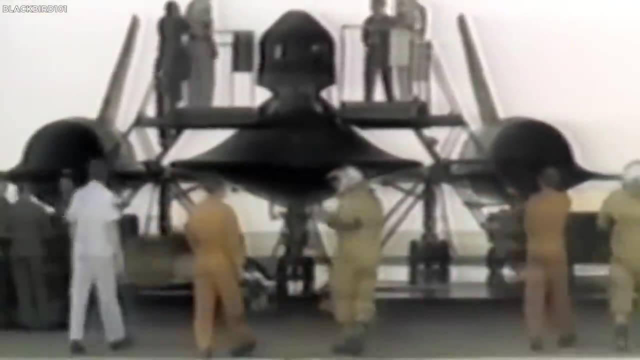 It's still considered by many as the most advanced aircraft of its type, flying at three times the speed of sound, faster than any weapon that could be fired at. The US tasked Lockheed with building what was then an impossible war machine after the 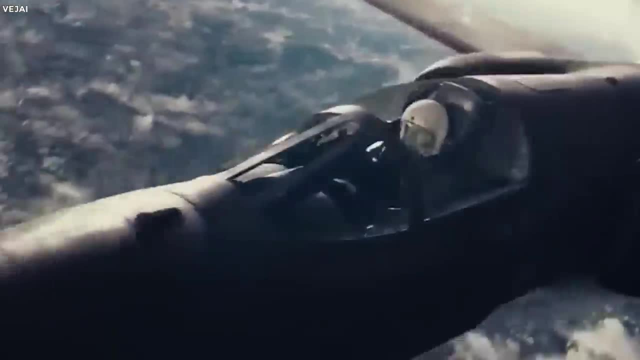 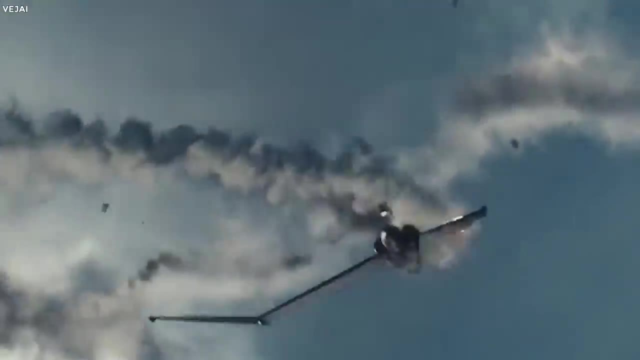 Soviets hit Gary Power's U-2 aircraft with surface-to-air missiles. The doomed plane fell from 70,000 feet to 30,000 feet before Powers could release himself and bail out of the damaged cockpit. However, during this period, Lockheed's advancement development group. 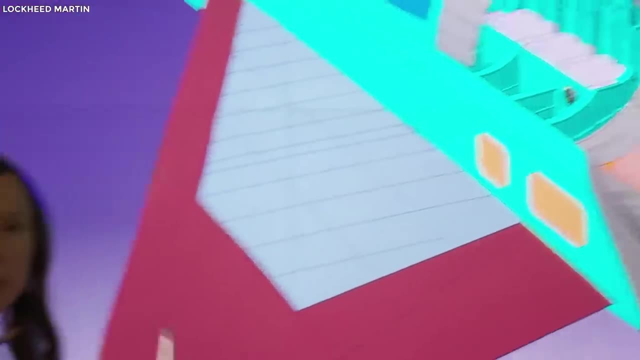 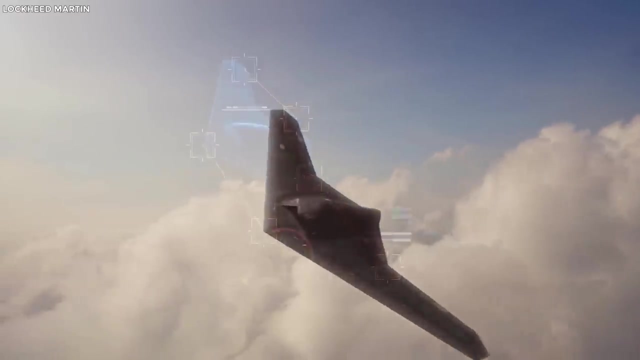 The Skunk Works in Burbank had begun working on an innovative craft to improve intelligence gathering, one that would fly faster than any aircraft before or since, at greater altitude and with a minimal radar cross-section. In other words, the engineers were building an aircraft. 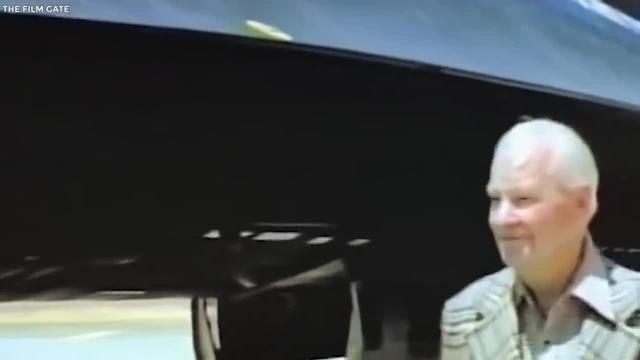 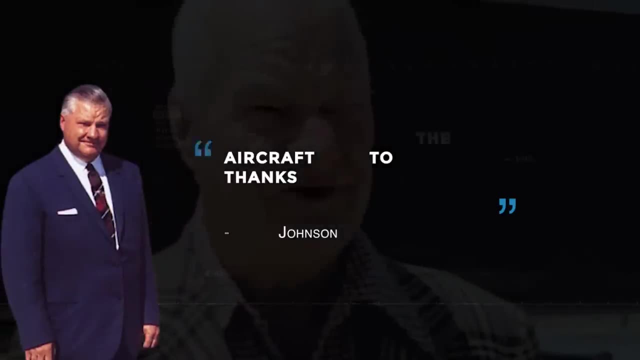 that could not be shot down. One of the most respected aircraft engineers that worked on the Blackbird was Kelly Johnson. He said everything about the aircraft had to be invented thanks to possible requirements. For example, the speed of the new aircraft was to exceed 2,000 miles per. 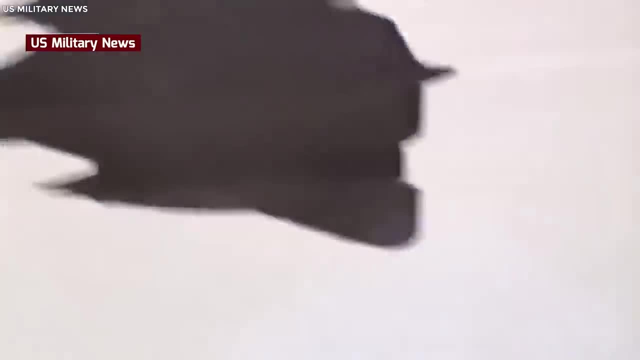 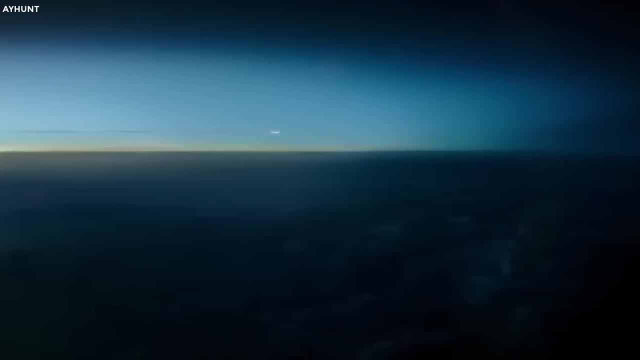 hour. Other planes of the era could reach that speed. however, they could only do so in short, afterburner-driven bursts. The new aircraft had to maintain this extreme speed for hours at a time. Other aircraft with conventional airframes would melt at this speed because the friction with the 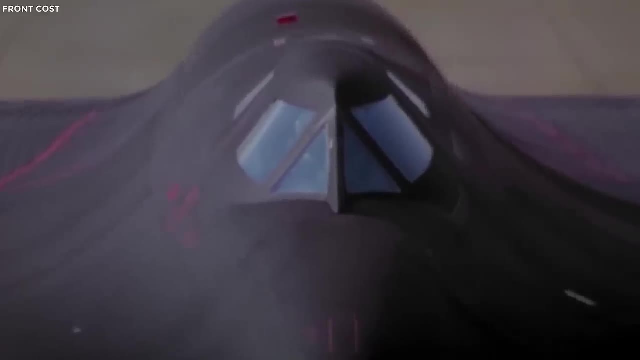 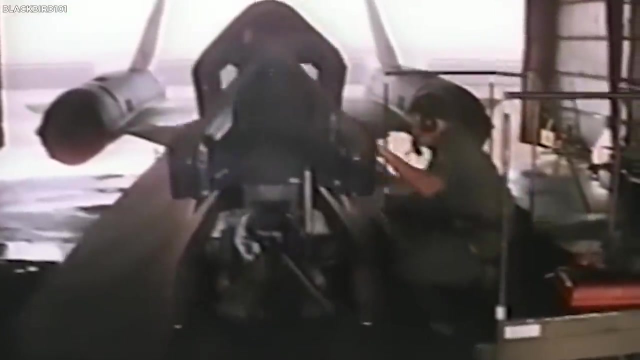 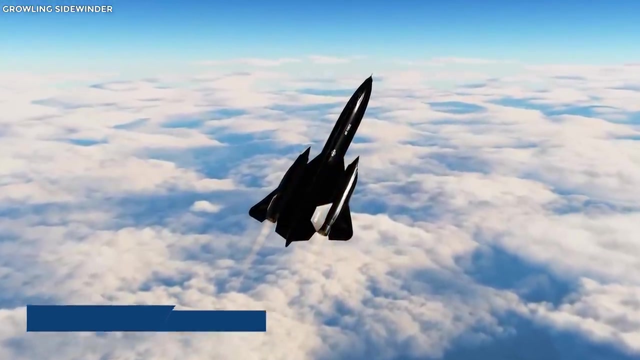 atmosphere generates plenty of heat. However, the Blackbird delivered on its responsibilities as the US military used it extensively for mission-critical reconnaissance for decades, until its official retirement in 1998.. Lockheed has the same primary mission with the SR-72, nicknamed Son of the Blackbird. 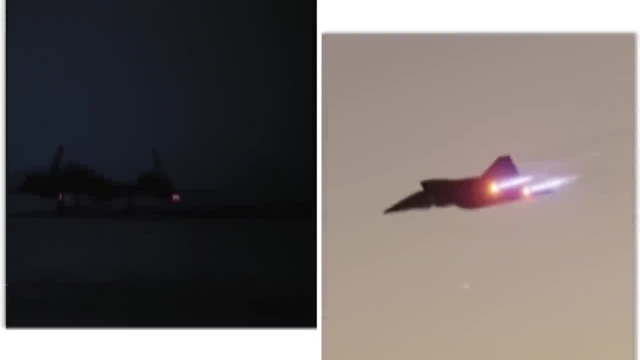 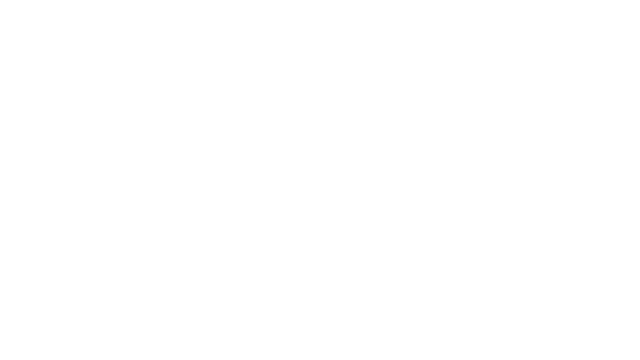 The aircraftmaker unveiled it in November 2013.. However, there is a huge difference between the SR-71 and SR-72.. The new Blackbird has an option of being unmanned, meaning the military will not put pilots at risk of the extreme conditions and dangers. 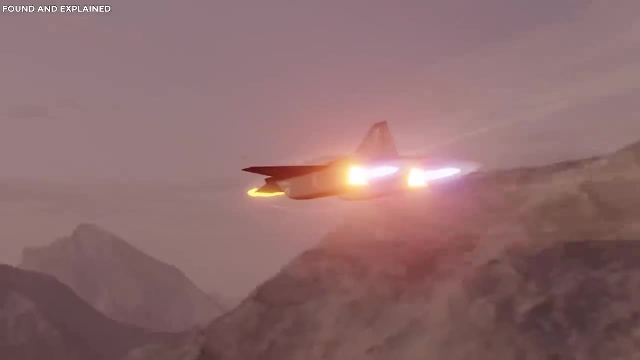 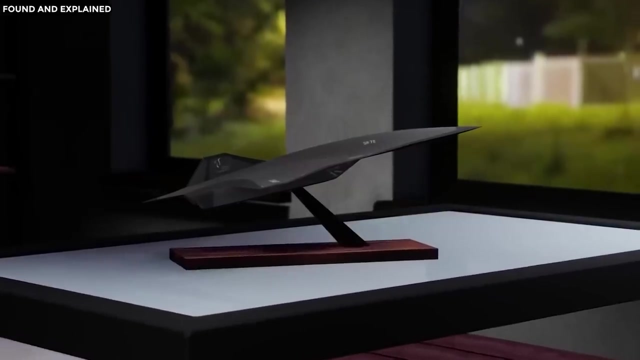 expected of its super high-speed, high-altitude flight with the SR-72,, which is designed to reach speeds around Mach 6.. The SR-72 is also designed to outrun any intercepting threats from the ground. The development has not come easy for Lockheed. 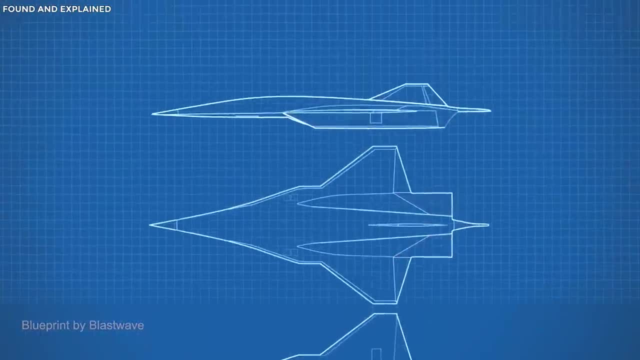 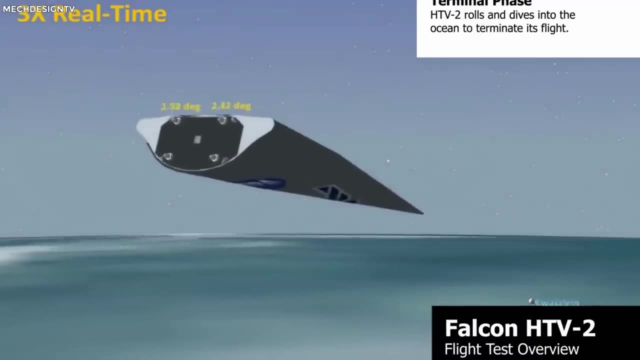 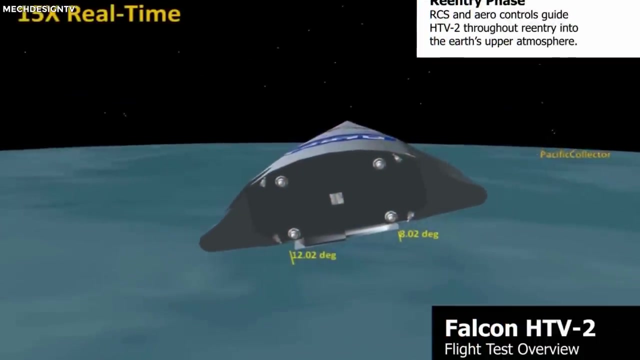 as it made several unsuccessful attempts and had to wait for some of the technologies it needed to develop. One such technology was the Hypersonic Technology Vehicle-2, or HTV-2, as part of the Defense Advanced Research Projects Agency's DARPA Falcon Research and Development Project. The HTV-2- 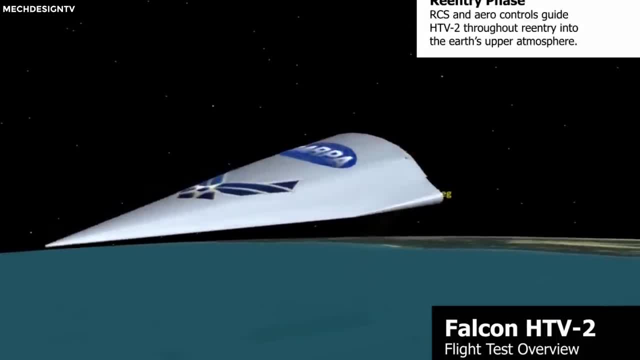 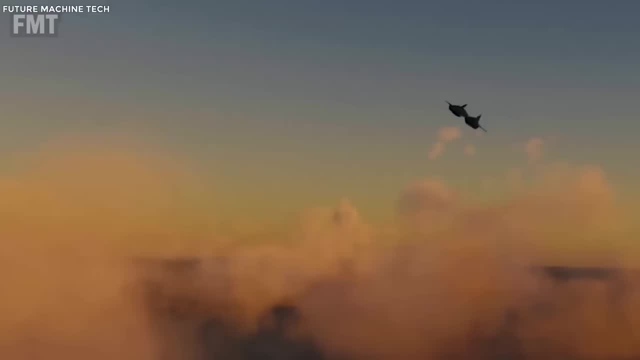 helped Lockheed in the collection of data on air and ground. Lockheed was also the first company to develop an aerodynamics, aerothermal effects, guidance, navigation and control. The HTV-2 had its first flight in April 2010, and the second more than one and a half years later. It achieved 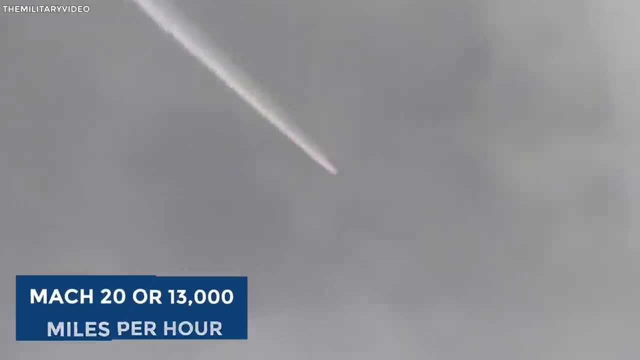 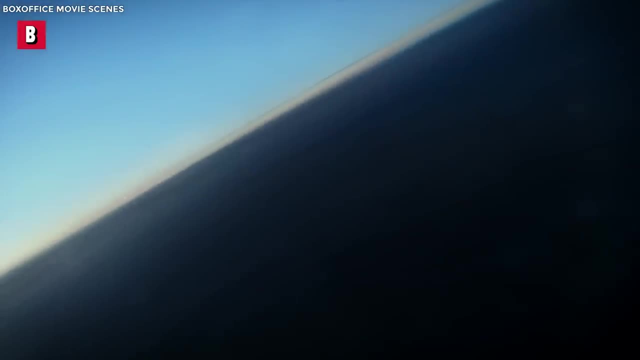 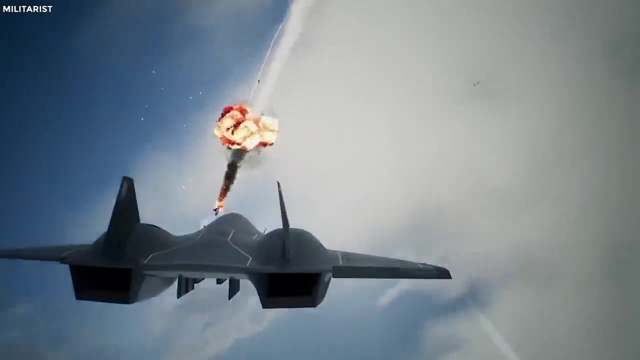 a maximum speed of Mach 20, or 13,000 miles per hour. The experience and data obtained from the HTV-2 helped Lockheed to materialize better design for the SR-72.. The SR-72 is a hypersonic reconnaissance aircraft with a similar size and range as its successor. It will hit targets. 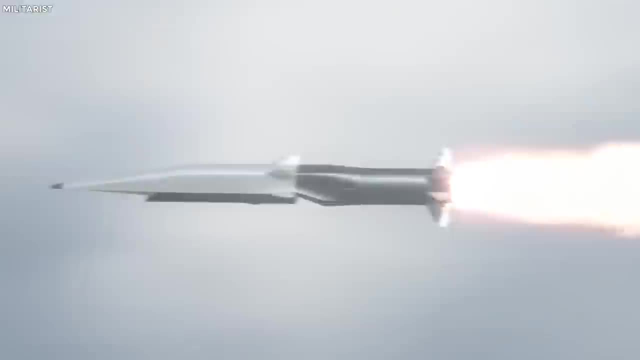 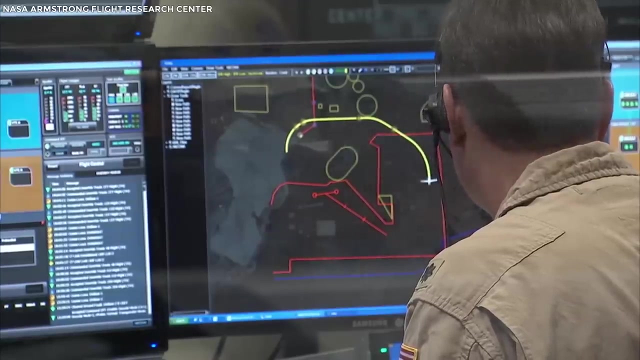 across the continent in less than an hour. when equipped with hypersonic missiles such as Lockheed Martin's high-speed strike weapon HSSW, The high speed of the aircraft ensures penetration into protected enemy airspace. It will be able to defy conventional air defenses. 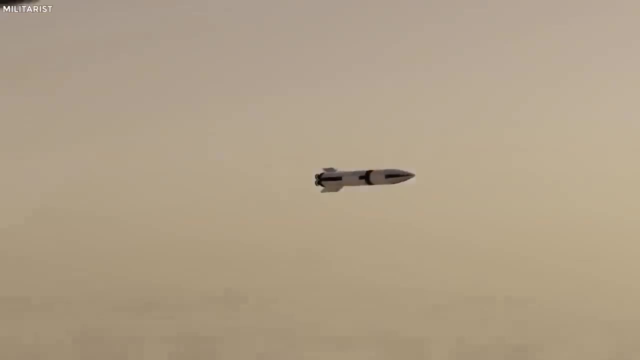 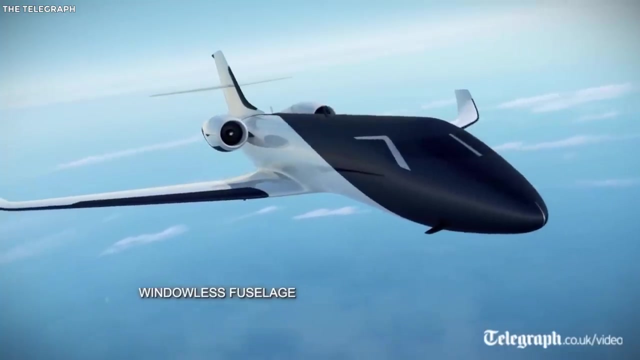 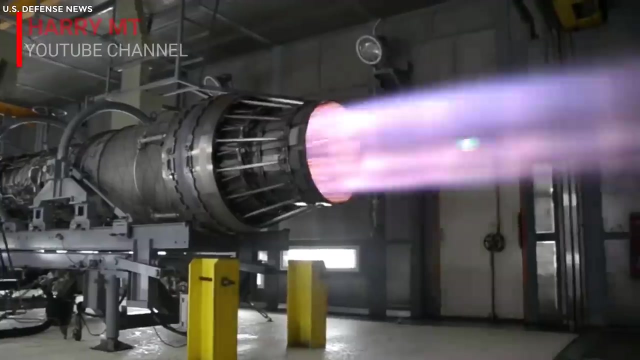 swoop in from extremely high altitudes and launch its payload before even being noticed. But in addition to that, the technology from this military project could have a revolutionary impact on future passenger airline travel between significant hubs. The SR-72 unmanned aircraft was designed to be able to operate the first ever jet-powered aircraft in the history of the 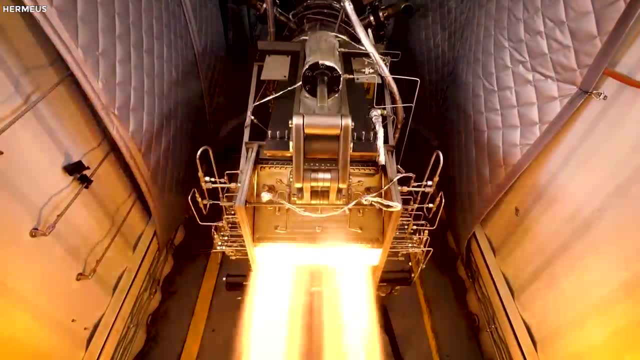 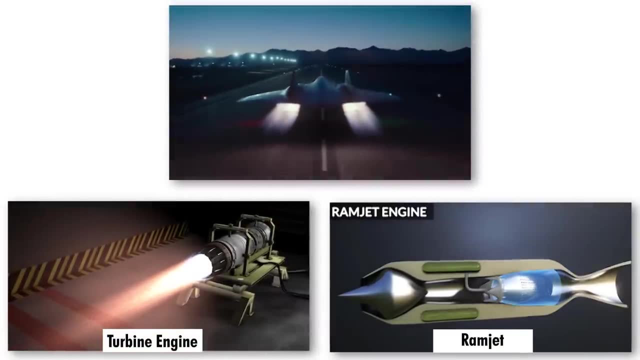 Soviet Union. The engine is powered by a small-capacity turbocharging engine that drives power from two sophisticated engines. It receives thrust from the turbine engine until it reaches a speed of Mach 3.. And the dual-mode ramjet will provide a boost to hypersonic speeds. 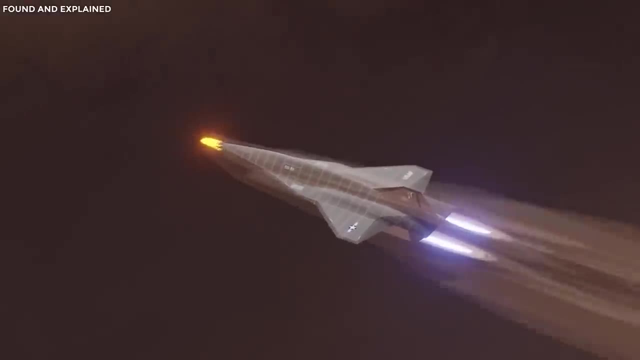 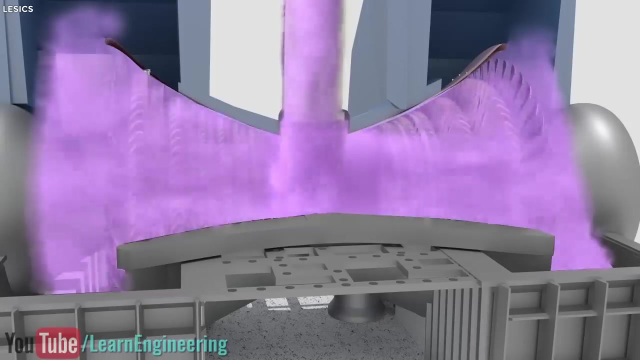 The aircraft will use a single inlet nozzle for both the turbine engine and ramjet to reduce the drag Skunk Works, teamed up with Aerojet Rocketdyne on the Turbine-based Combined Cycle. ground tests of the TBCC system were performed by integrating a small off-the-shelf turbine engine. 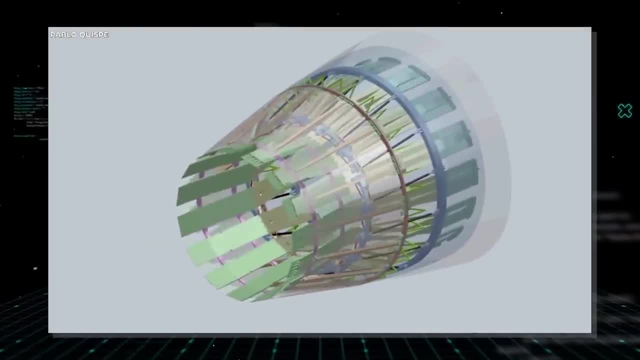 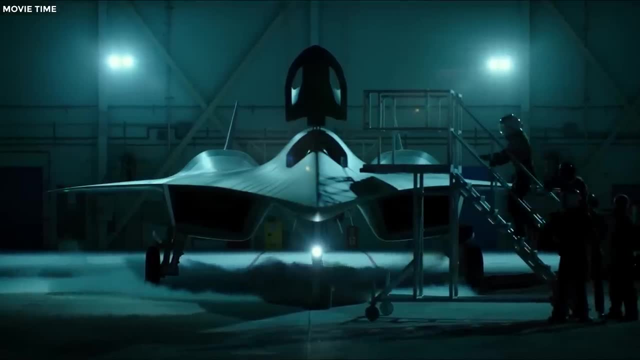 with a dual-mode ramjet-scramjet integrating an axisymmetric inlet and a nozzle. The SR-72 is already popular with aviation aficionados. Movie makers are also following its development closely, as the aircraft has been sported making a cameo in the trailer of Top Gun Maverick film In the 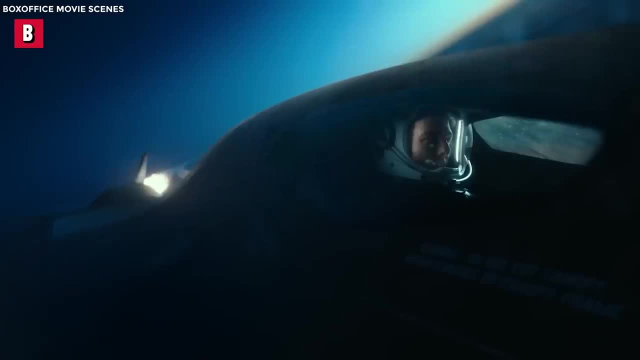 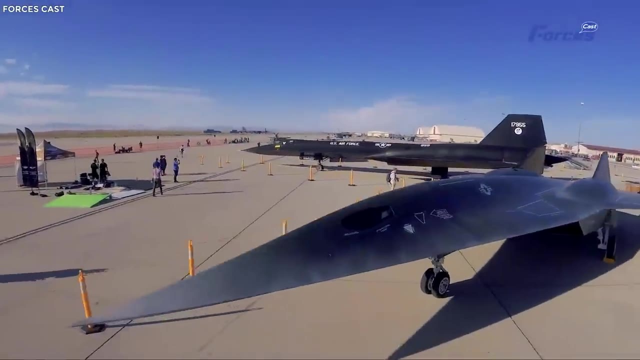 trailer, Tom Cruise's character Pete Mitchell, with call sign Maverick, can be seen piloting an experimental craft that looks suspiciously like a fictionalized variant of the SR-72.. The new SR-72 has also made an appearance in a short promotional video made jointly by the. 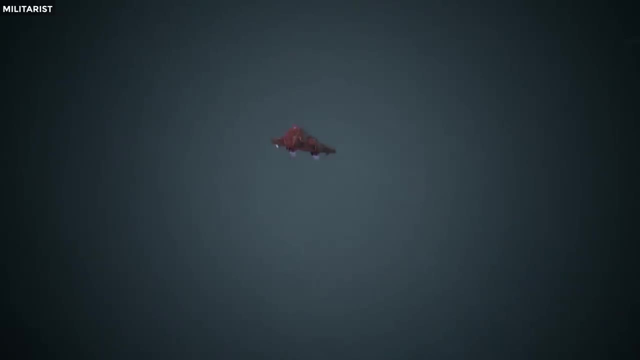 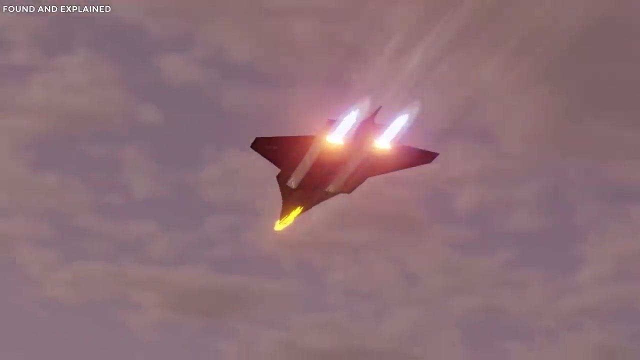 United States Air Force and Space Force. The aircraft shows up at the very end of the video and only an outline and a few details are visible. The object is most likely a computer-generated image or a mock-up, but if anything, it further removes doubt that the US military is working. 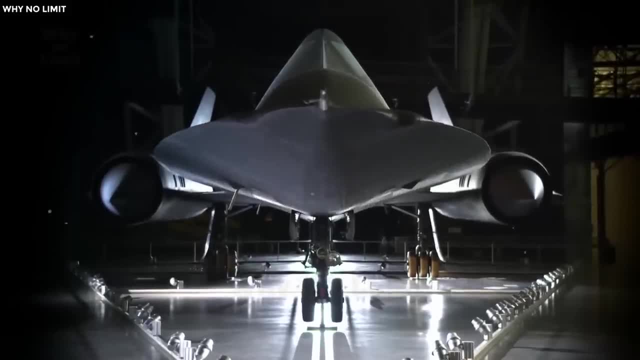 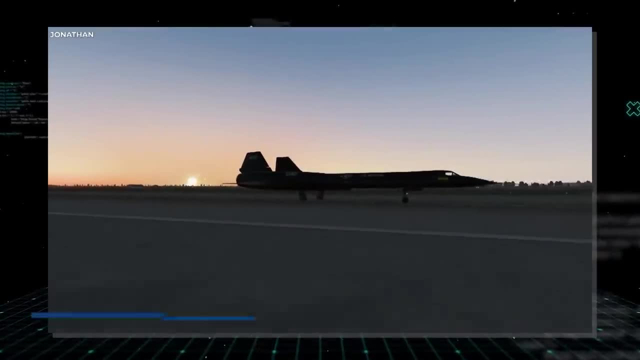 on the mysterious plane. Beyond videos, there have been reported sightings of the SR-72.. A source has revealed to Aviation Week that they spotted a small demonstrator aircraft landing at Skunk Works facilities in Palmdale, California. The demonstrator is said to be an unmanned subscale. 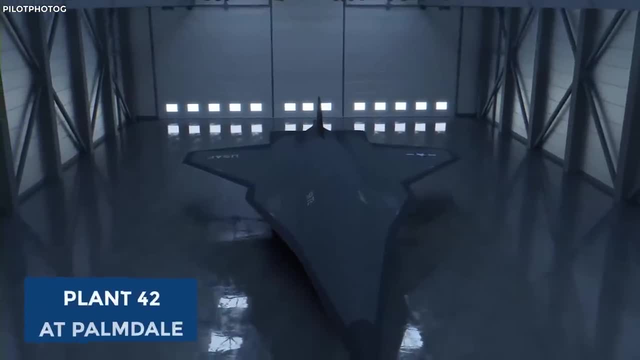 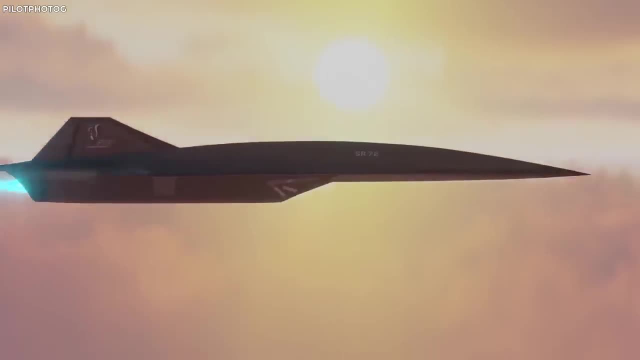 aircraft and was spotted flying into the US Air Force's Plant 42 at Palmdale. That's where Skunk Works is headquartered. The vehicle, which was noted landing in the early hours at an unspecified date in late July, was seen with two T-38 escorts. Lockheed Martin declined to comment. 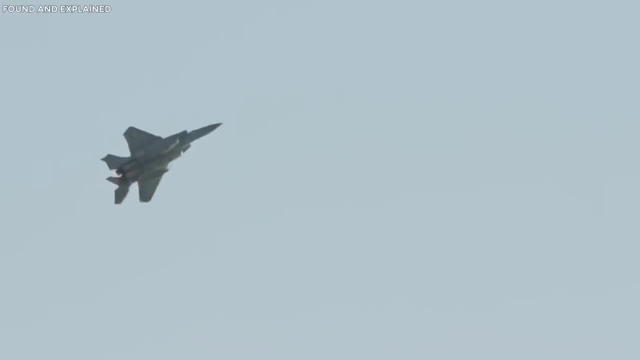 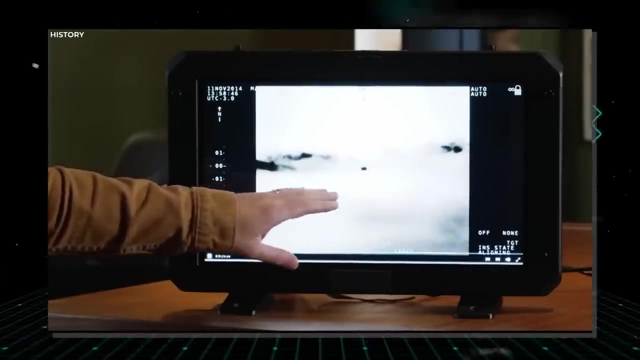 directly on the sighting. The sighting is not unusual, as classified military aircraft usually go through flight testing years before the details are made public. In other public sightings, fans have reportedly photographed the new Blackbird in Kansas where the mysterious flying object was spotted. The person that took the pictures explained: 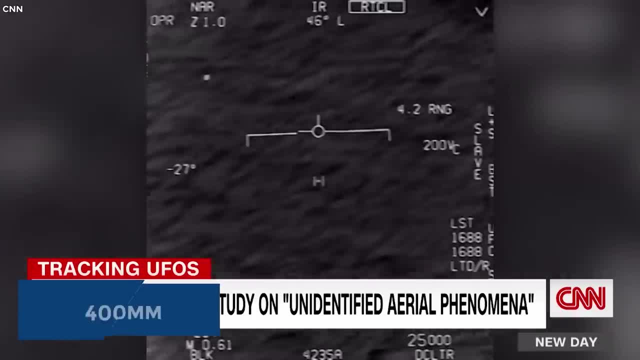 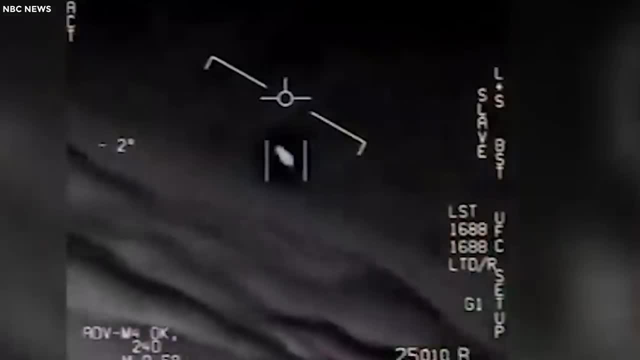 the photo is grainy because it was taken with a hand-held maxed-out 400mm telephoto lens through a cloud layer, after which it was severely cropped to bring it up even closer. He added that there are no way to judge its size, as there is no point of reference, But this was in addition to another sighting in Texas. This particular sighting was taken by the US Air Force, which is also known as the US Air Force. The US Air Force, which is also known as the US Air Force, is also known as the US Air. Force, The US Air Force. 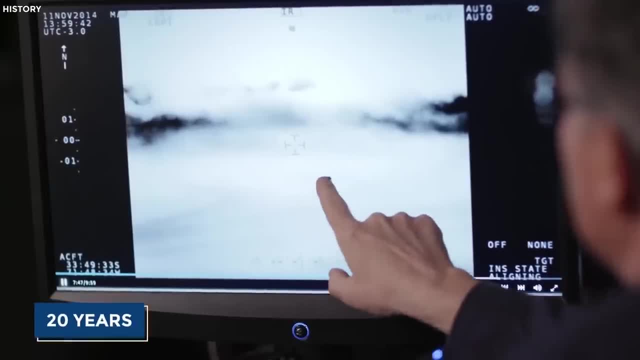 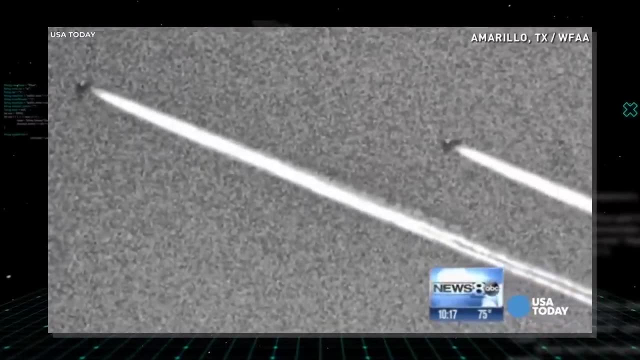 in particular. one was much more significant, as a retired Marine with about 20 years of aviation experience commented on it. The three aircraft were spotted flying over Amarillo and the pictures were posted online to help with the identification. The retired Marine, James Vinyard, told the Houston Chronicle that the three aircraft were the mysterious. 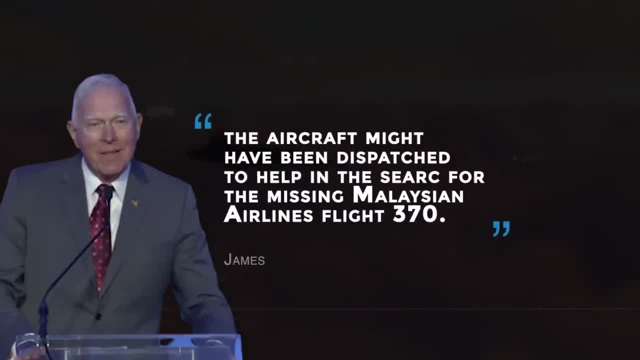 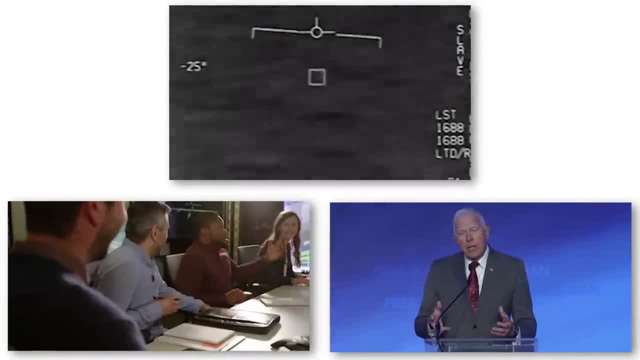 SR-72 Blackbirds. He claimed that the aircraft might have been dispatched to help in the search for the missing Malaysian Airlines Flight 370.. However, other experts disagree with him, pointing out that the aircraft was still in development. When will the new Blackbird? 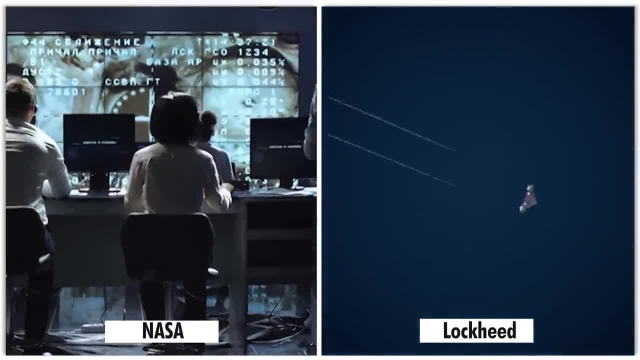 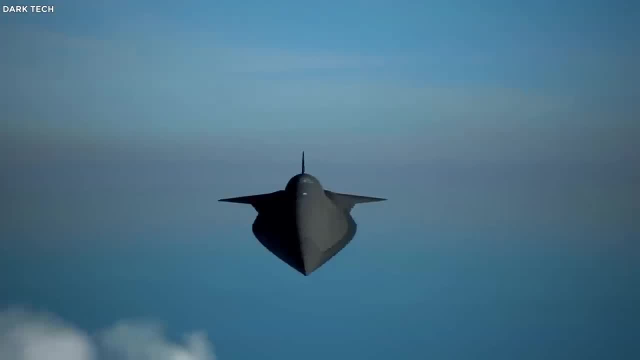 go into operation. NASA and Lockheed are keeping tight lips on this, and the silence is understandable, as it is a top-secret project. However, there are different estimates from different experts, but the consensus is that the aircraft may require a few more years before becoming certified. 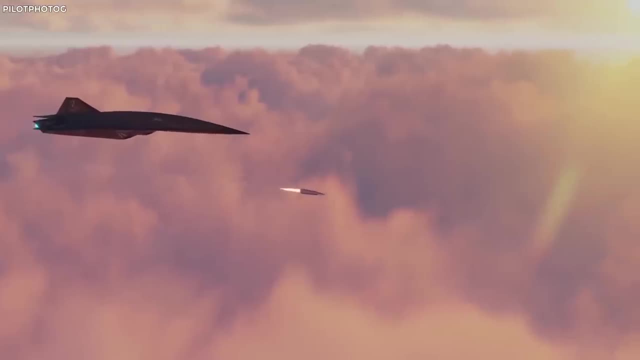 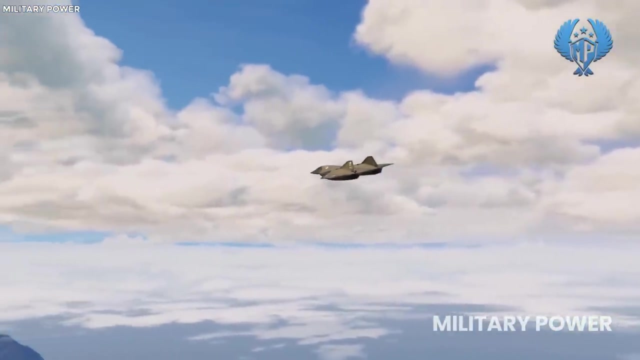 and it might be in the next decade that it will officially join the Air Military Fighting Fleet. We expect the number of sightings to increase as Lockheed tests the new aircraft. But that is not the only secret world powers are guarding. Take, for instance: 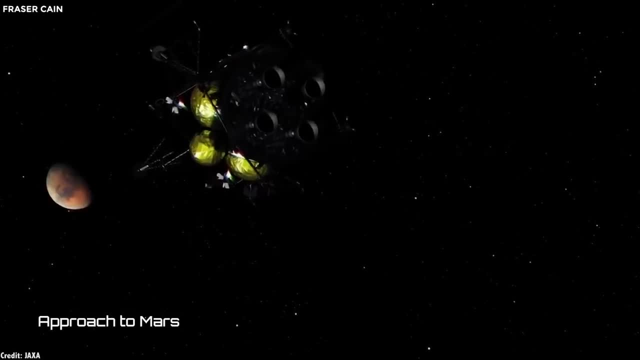 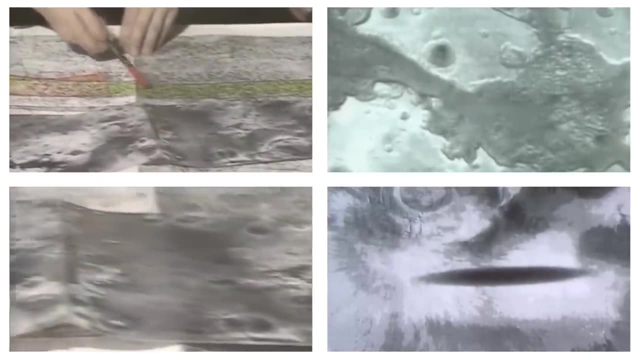 the Russian Phobos mission to Mars. The mystery of the two probes may never be solved completely, as the two probes are lost to us forever. However, before completely going offline, one of them managed to send back a collection of 38 images, and some of them will forever. 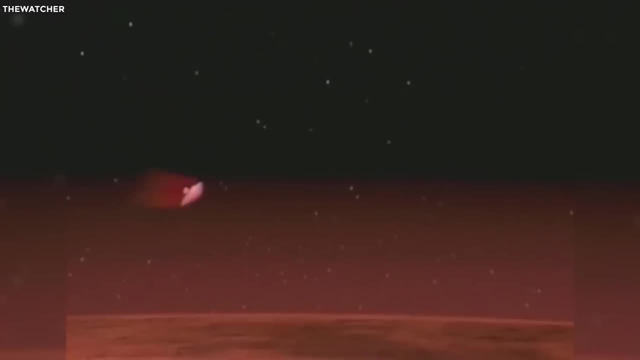 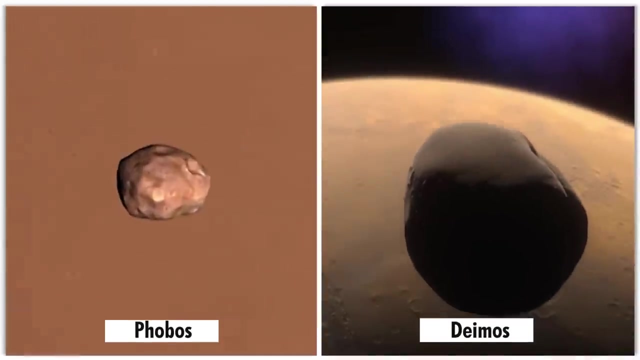 haunt us because of their content. Analysists believe the probe had an extraordinary encounter before going off. The Phobos mission planned to put two probes on Mars to study the planet and its two moons, Phobos and Deimos, but with the emphasis on the moons, Phobos was particularly 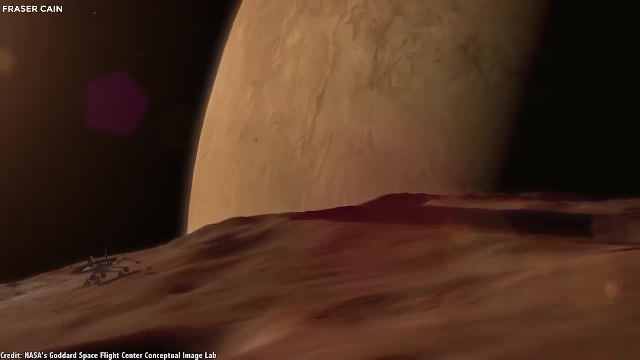 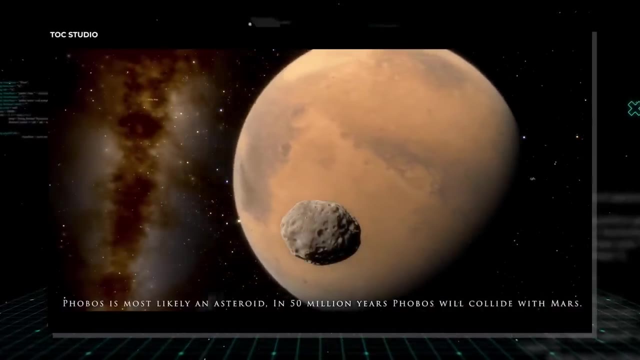 attractive to the Russians Because its orbit required a relatively easy approach for a Mars orbiter powered by traditional chemical rockets. In addition, Phobos, with its projected low mass relative to its size, inspired a prolific Soviet astrophysicist, Isov Shkolovsky, to hypothesize in the popular press. 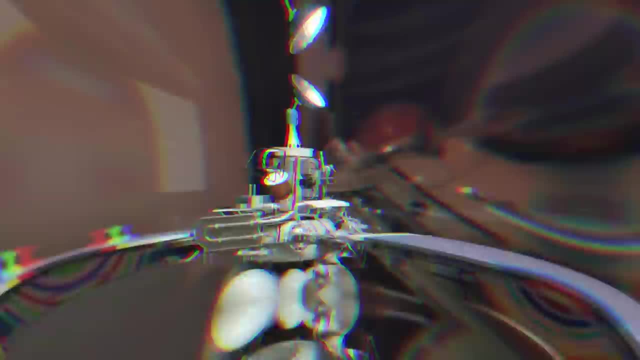 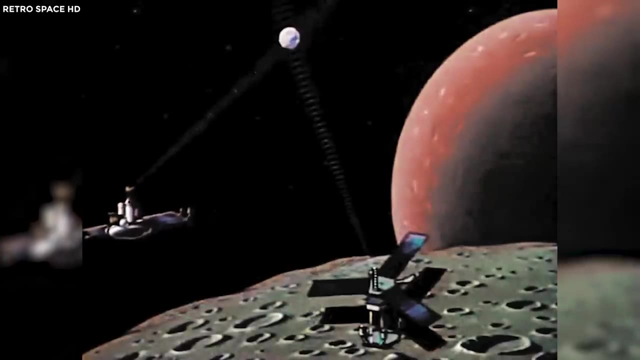 that the moon might be hollow and even of an artificial origin. However, only one probe, Phobos 2, made it to the planet. Phobos 1 operated with no issues until an expected communication session did not occur. Try as hard as they could. 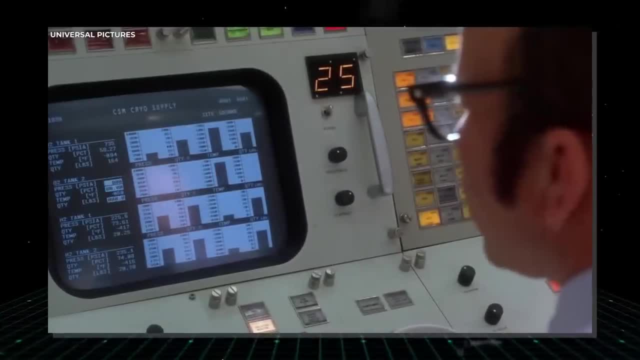 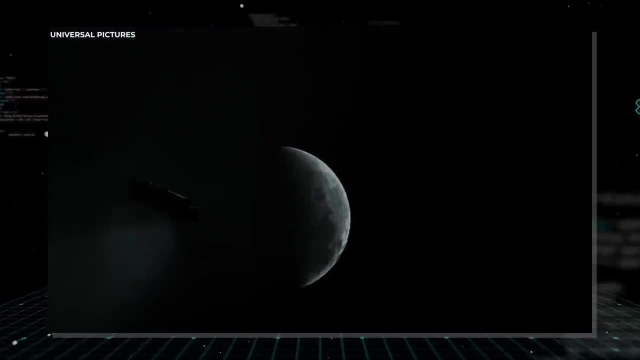 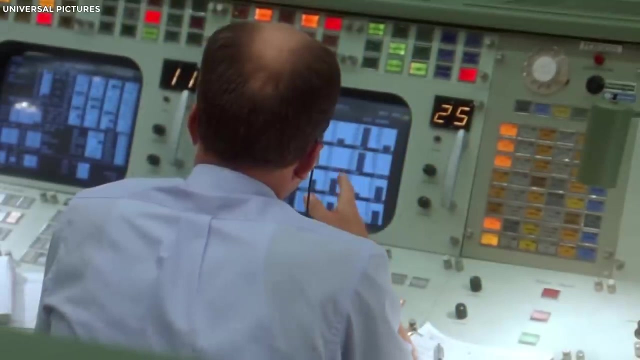 controllers could not regain contact with the spacecraft. The problem was traced to a problematic software update that deactivated the altitude thrusters. This prevented the spacecraft from maintaining its lock and the spacecraft could no longer appropriately orient its solar arrays, thus depleting its batteries. Software instructions to turn off. 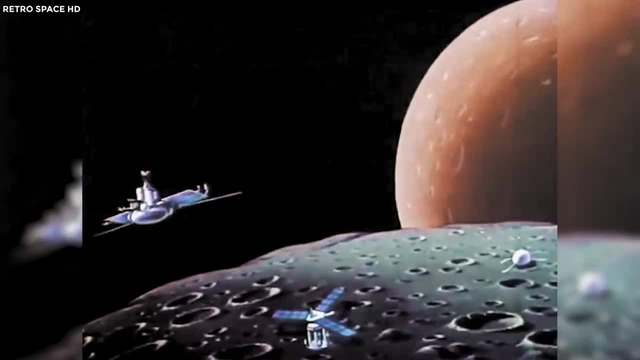 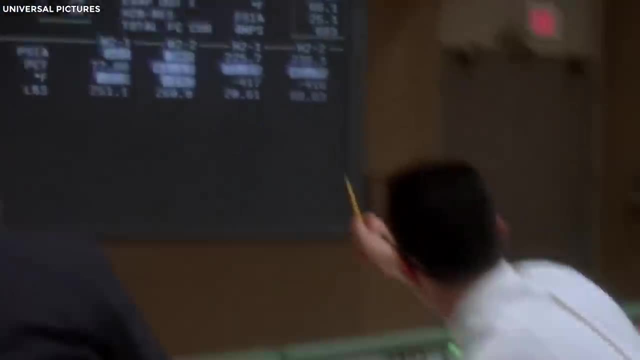 the probe's altitude control- normally a fatal operation- were part of a routine used when testing the spacecraft on the ground. Normally, this routine would be removed before launch. However, the software was coded in PROMS, so removing the test code would have required removing and replacing the entire 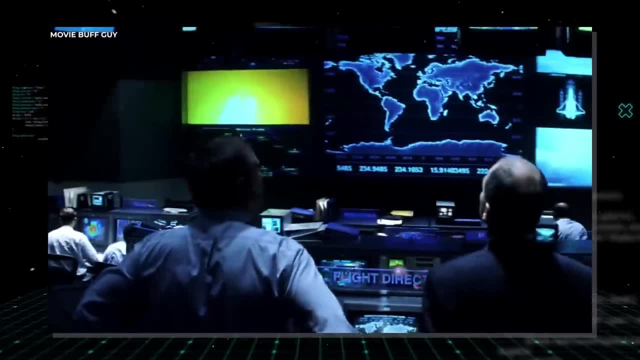 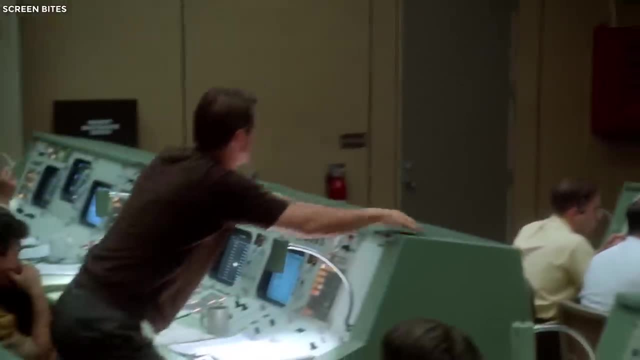 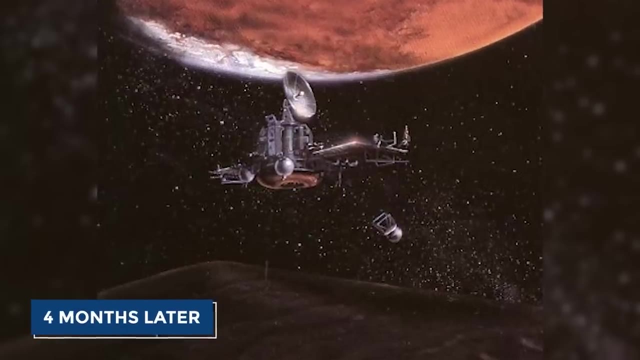 computer Facing lots of pressure due to the short time before launch, the engineers were forced to leave the command sequence in, even though it should never happen. However, a single character error in constructing an upload sequence resulted in the command executing and the Russians lost the spacecraft forever. Phobos 2 launched about four months later. 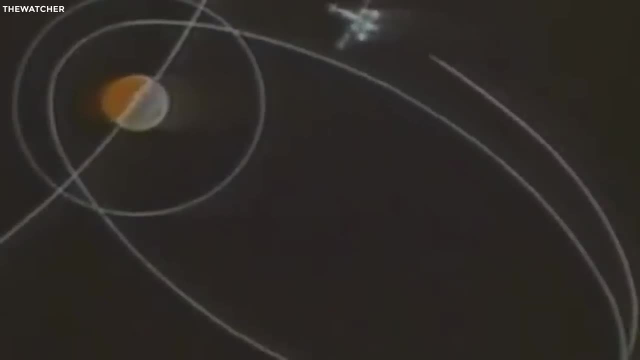 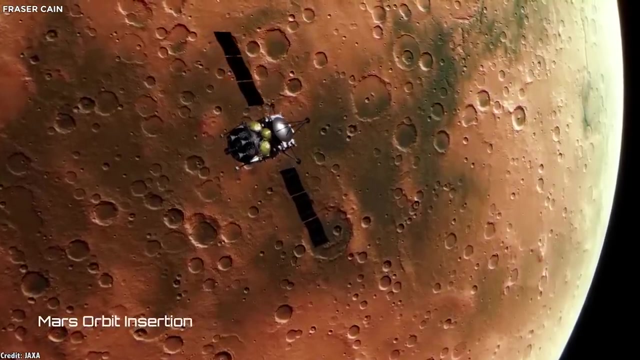 and this is where the plot thickens. The aircraft did behave as the Russians expected, much to their relief for the whole of the trip to the red planet. That took a whole year before it was ready for orbital insertion. However, it managed to gather. 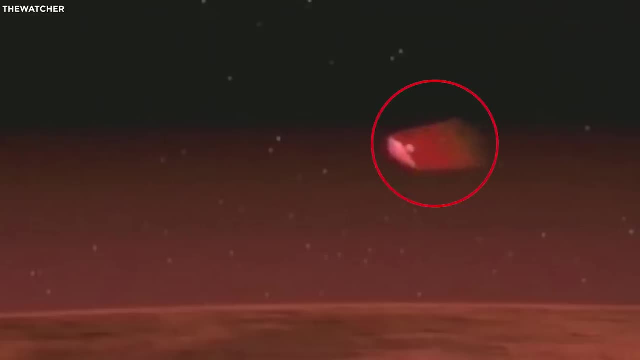 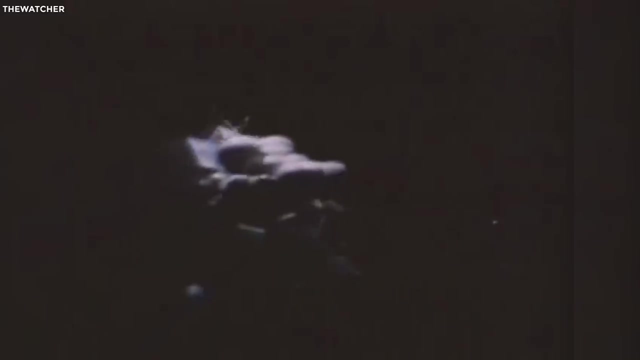 some data before its own tragedy occurred. a few days before it was scheduled to land, A strange event caused a critical failure. The mission controllers desperately tried to regain communication with their malfunctioning spacecraft for many hours, but nothing worked. The leaders of the mission tried to cover up the failure and the few photographs that Phobos 2. returned, but leaks always happen and some Soviet agents actually came forward with official evidence and conclusive mission data. Thankfully, Russia's hard luck did not stop other space agencies around the world from funding extraordinary experiments, including hugely successful missions like the Mars Global Surveyor, Mars Express. 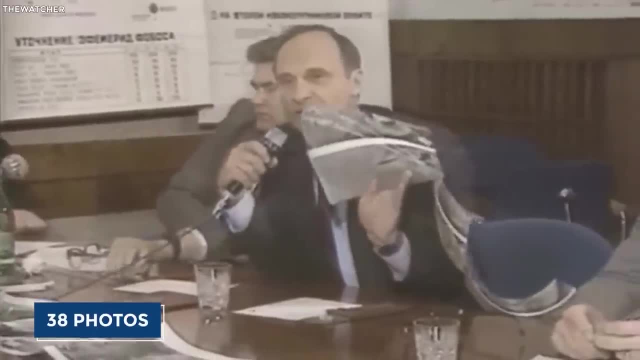 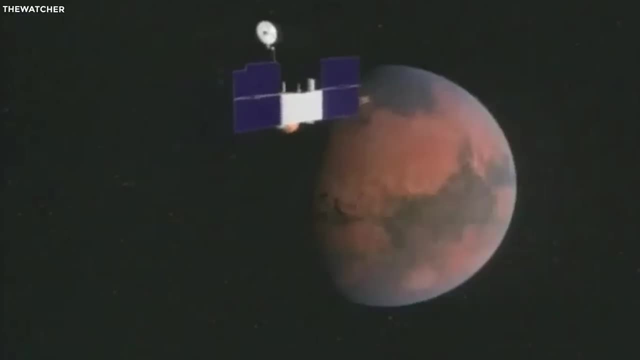 and Mars Reconnaissance Orbiter. However, the Russians have 38 photos, some of them with very sharp resolutions, to show for their effort. But what was unusual about the images that Phobos 2 sent back to the Russians, And why did they try so hard to conceal it? One of them contained what? 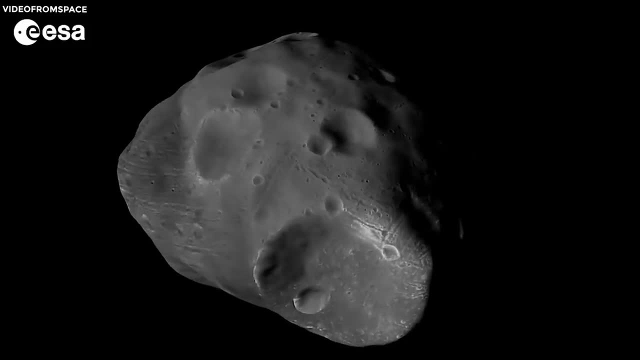 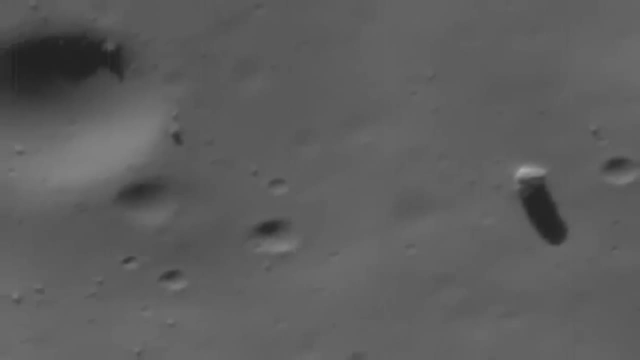 is now known as the Phobos Monolith. It is actually a large rock on the surface of Mars' moon Phobos In size it's about 85 meters across. Monoliths are not an unknown phenomenon. A monolith is a geological feature. 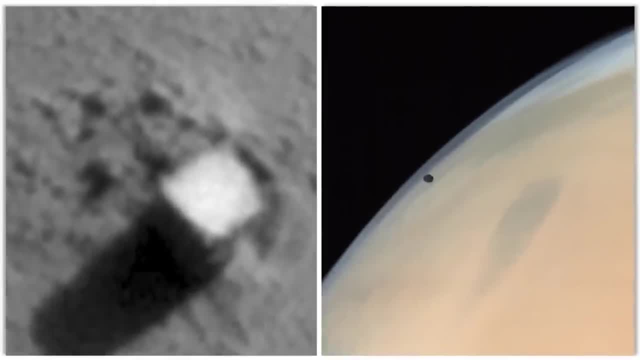 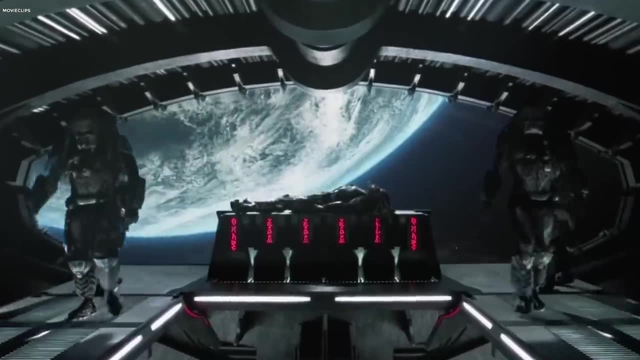 made of a single massive piece of rock, and you can find monoliths naturally occurring on the Earth. However, looking at this one in the pictures, it says some of the hallmarks of being artificial, which could only suggest one thing: It was placed there by aliens. 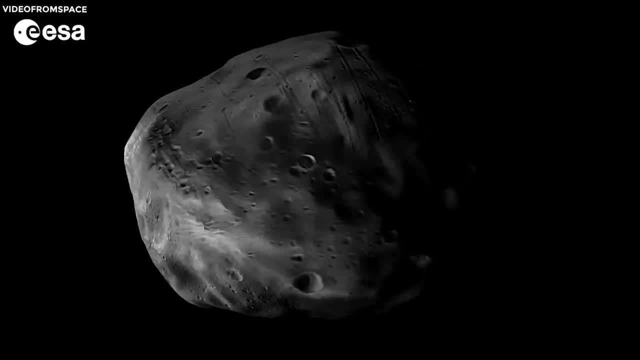 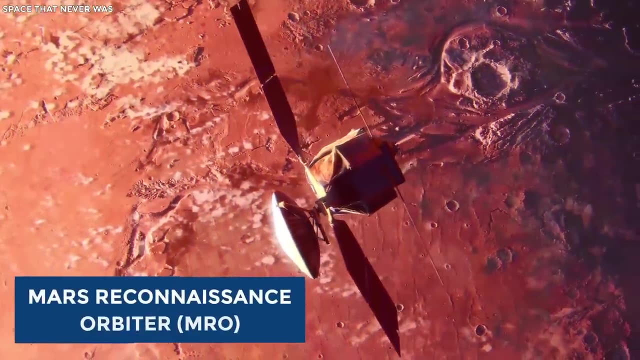 The monolith is a bright object near the Stickney Crater, described as a building-sized boulder. In the glare of the sun, this mysterious object casts a prominent shadow on the moon. When the Mars Reconnaissance Orbiter spacecraft was mapping Phobos, the moon, and sent images, UFOlogists were surprised to. 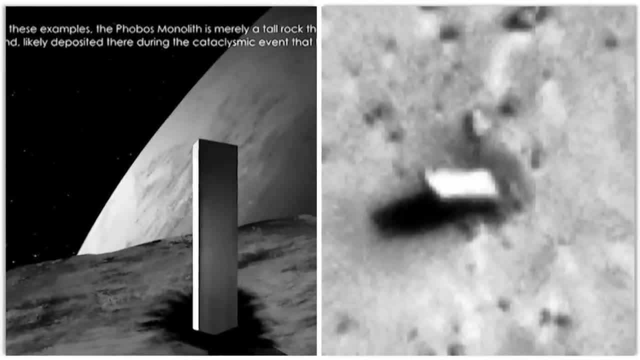 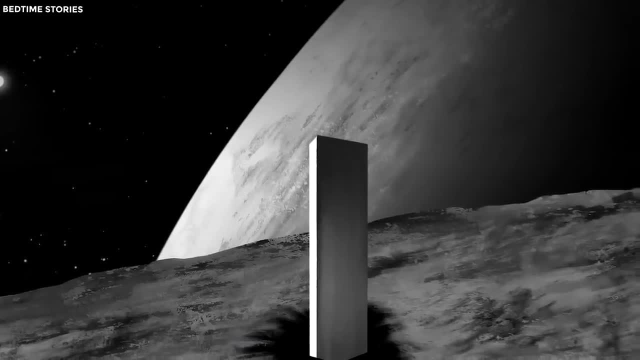 confirm the monolith was still standing and still looked as artificial as it did in the Phobos 2 photos. One of the things that made the monolith eerie was the sense of isolation. It was just standing there in plain view, a large rectangular object, like in the middle of nowhere, Nothing in. 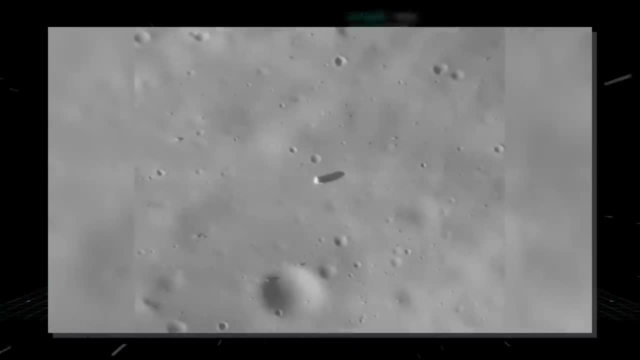 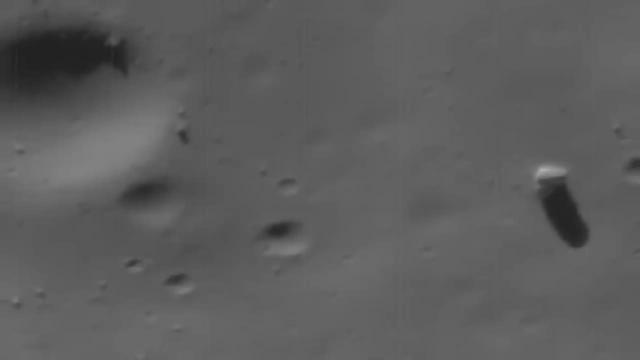 its immediate surrounding was similarly shaped or sized. However, as lonely as it stood, it was hard to imagine it got there by chance And to this day, the questions such as what exactly it was its purpose and who placed it there have not been successfully answered. 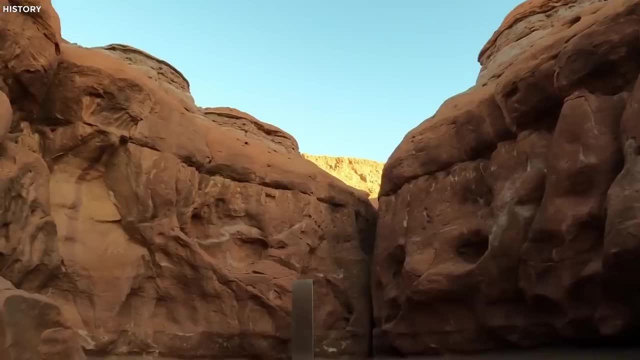 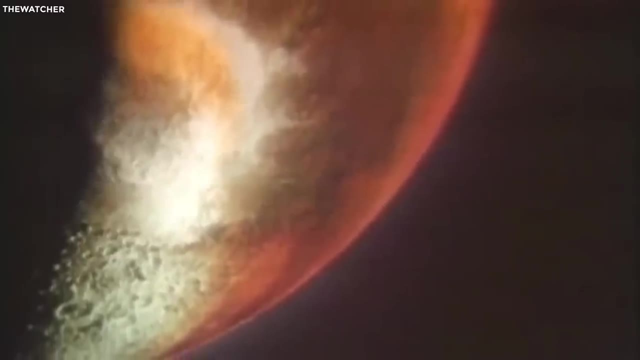 And when there are no clear-cut answers, you can bet humans are creative enough to come up with suggestions. For example, some Martian scientists have suggested the monolith was a result of accumulation of particles over the millennia, Although just how it got the perfect shape? 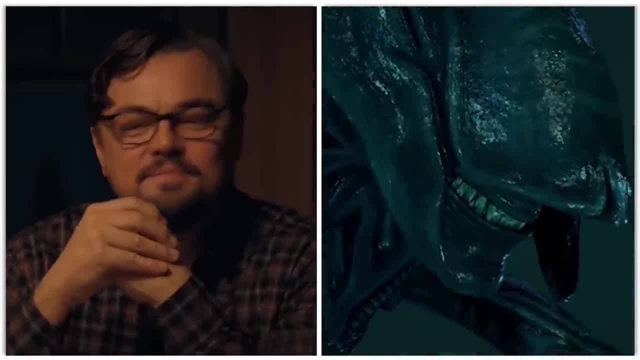 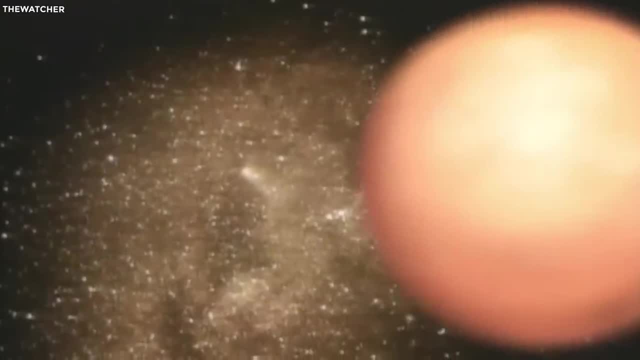 remains a difficult nut to crack, But it's more tempting to believe that this was the handiwork of aliens. Famous scientist Dr Isaac Asimov penned a story that suggested that the Phobos moon itself was a giant alien ship That was abandoned and trapped in orbit around Mars by gravity. However, the Phobos mission was. 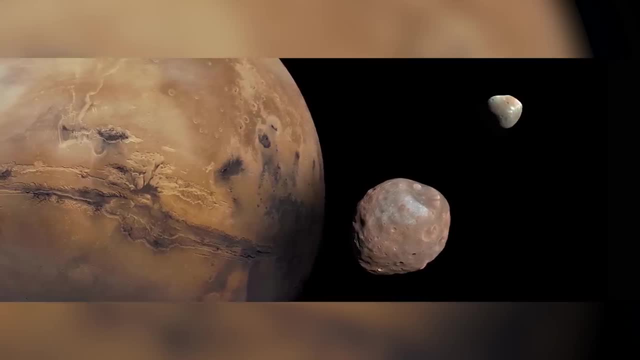 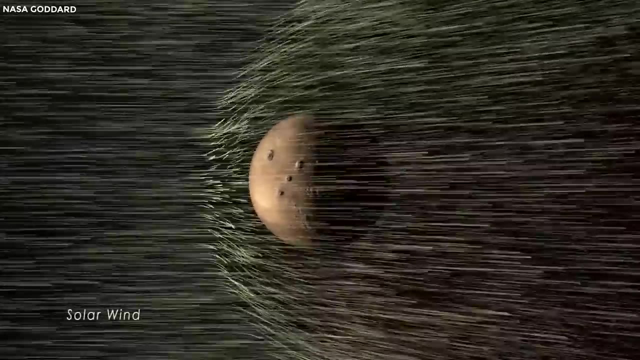 not a complete failure for Russia, for multiple reasons. Apart from getting photographs of one of Mars' moons, scientific data from the mission helped them confirm a theory that potential Martian water was blown away by solar wind. Yes, the red planet used to have water, but the solar 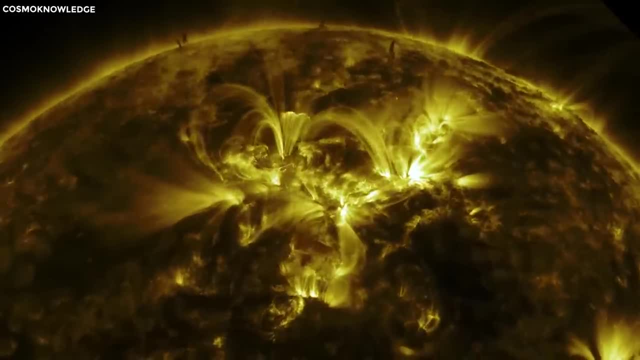 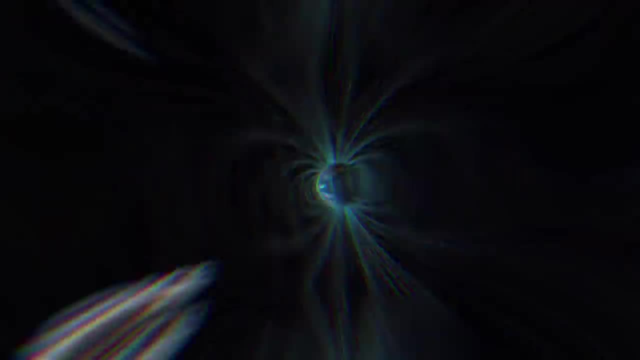 wind took it all away. Interestingly, solar winds could not be stopped because Mars did not have a magnetic field. This means the Earth could have lost its water too, save for its own magnetic field. In addition, some previously unseen areas of Phobos were covered in the few photographs. Phobos 2.